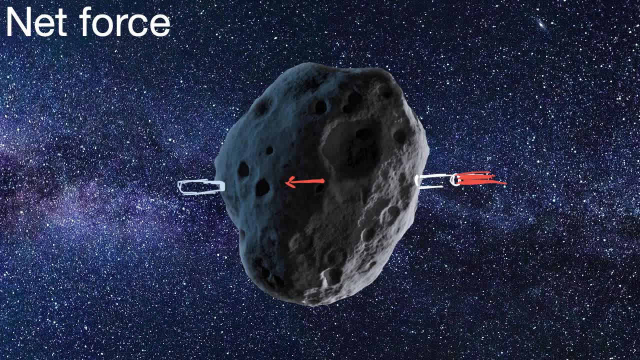 on this side of the asteroid, And y'all ignited it at the exact same time, So this one is going to push in the other direction. What do you think is going to happen if these happen at the exact same time, Even though there's now twice as much force? 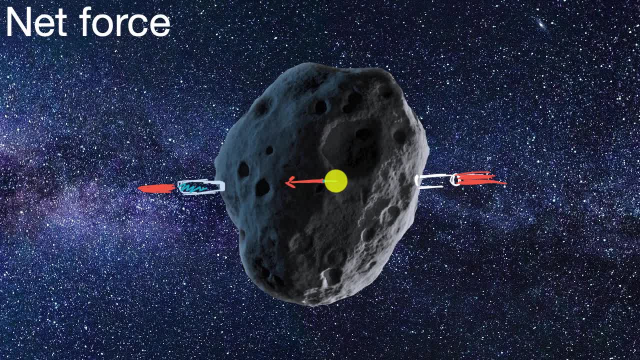 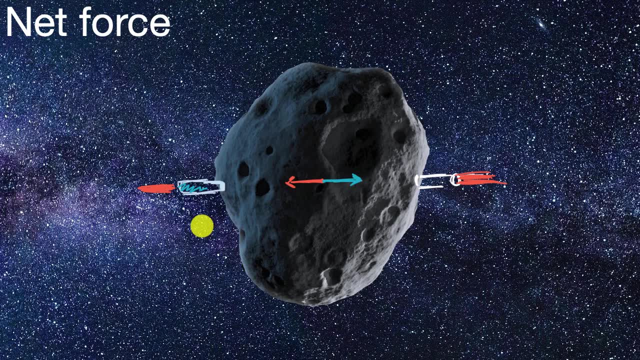 being exerted on this asteroid. it's going in opposite directions, So they zero out, and so there's zero net force, And so this asteroid won't be accelerated at all. Now let's say that a third friend wanted to correct this situation. 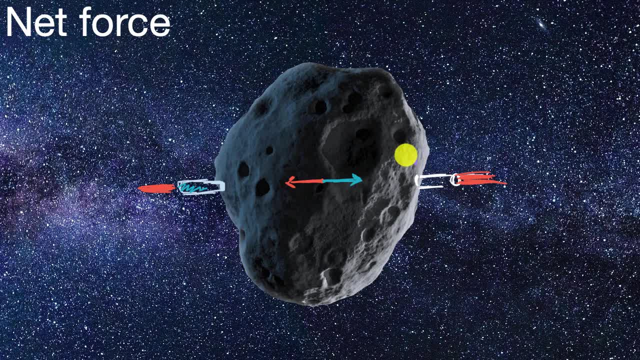 And this isn't necessarily the most efficient way, the most efficient way to do it. But what they do is they put another identical rocket right over here And, let's say, ignite that. Now what will happen? Well, now you had the original two forces. 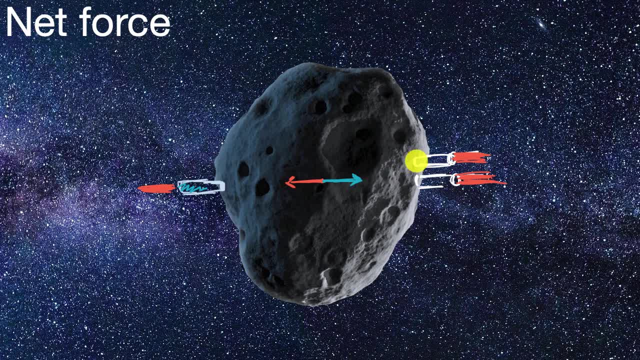 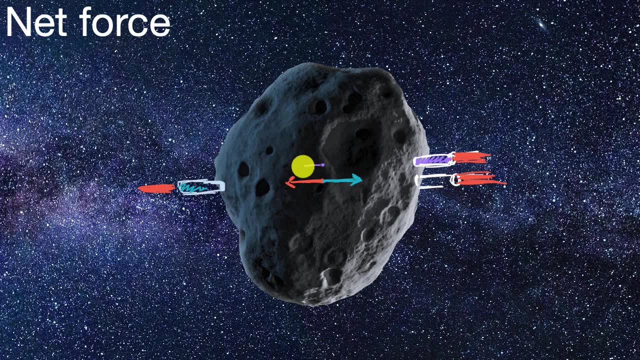 that net out to each other. but now you have this also, this new force which I will make in purple, because it's a purple rocket, And so that new force you could draw like this to show: all right, that will now be the net force. 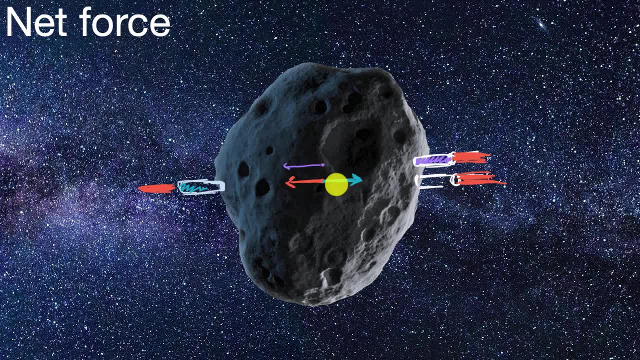 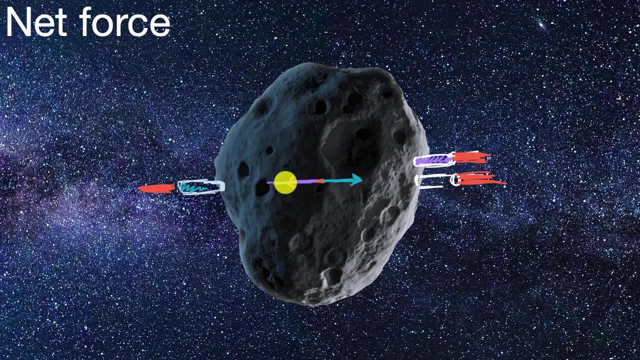 Because you have the equivalent of two rockets going in the left direction and one rocket going in the right direction. Or another way we could draw, that is, we have two rockets going in the left direction, So that would have a force that looks like this: 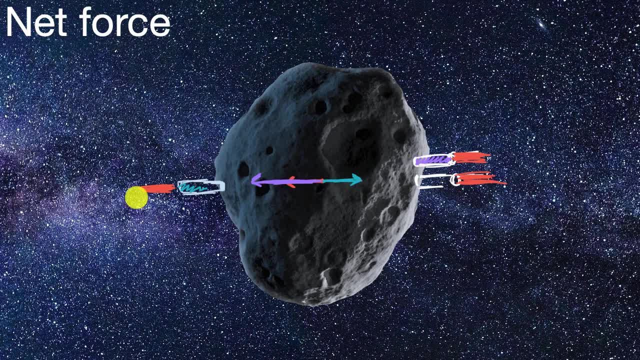 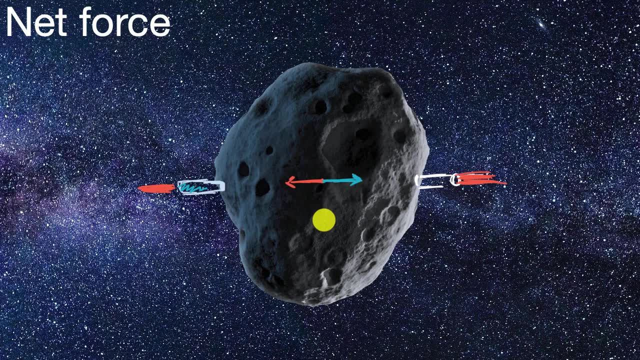 And then we have one going in the right direction, And so, if you were to net it out, this is equivalent to just having one rocket that we originally saw. That's equivalent to just going back to what we originally saw. So the important takeaway: 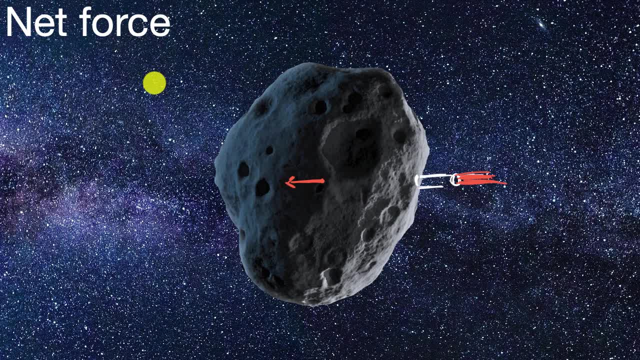 from this video is that it's not just about the force that's being applied. If you want to think about how something might be accelerated and in what direction, you need to think about the net force, because some of the forces could counteract each other.